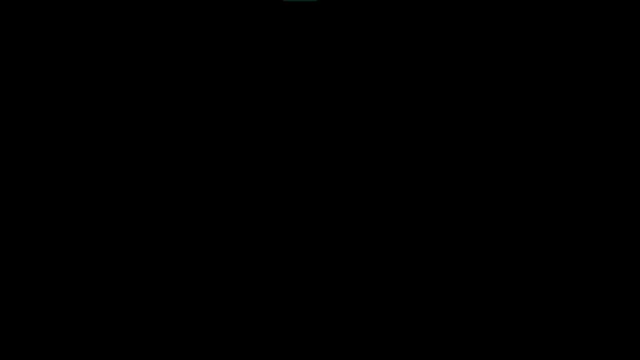 and that there was a pattern for which words a language had Words for brown, purple, pink, orange and gray were never present in languages that didn't already distinguish between green and blue. They broke this pattern down into a sequence: Purple, pink, orange and gray come. 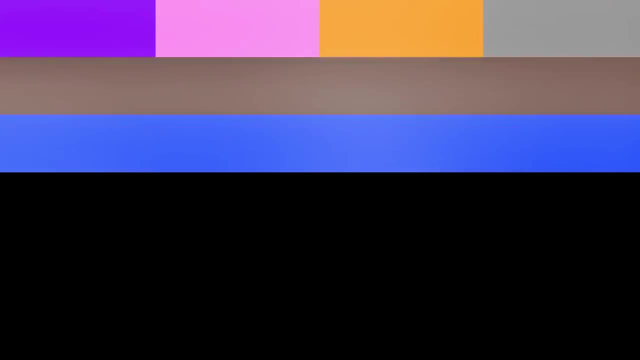 after brown. Brown comes after blue. Blue is perceived as a color. Blue is perceived as a color. Red is perceived as a color. Green is perceived as a color. Green is perceived as a color Green. and yellow come after red And finally, the most basic language categories are dark cool. 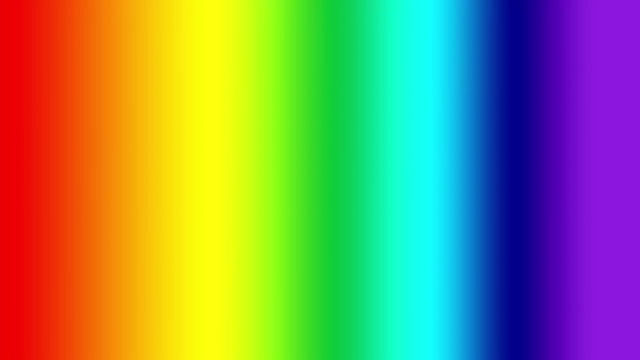 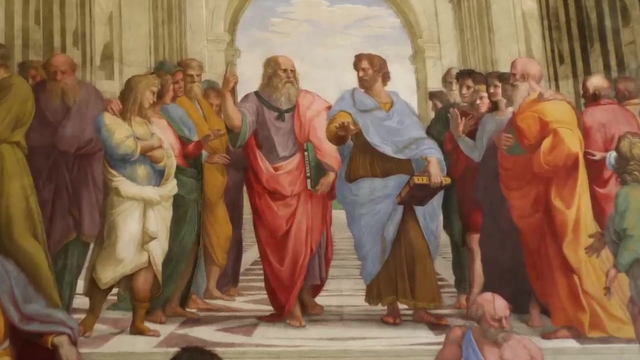 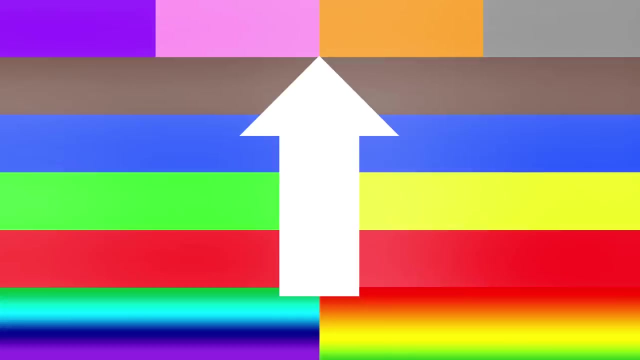 and light warm, encompassing the set of all cool colors and warm colors as two categories. Now it's important to mention that this study has been criticized. It assumes an ethnocentric bias based on western scientific and political thought. It's basically implying this idea of progress where more primitive cultures have not sufficiently 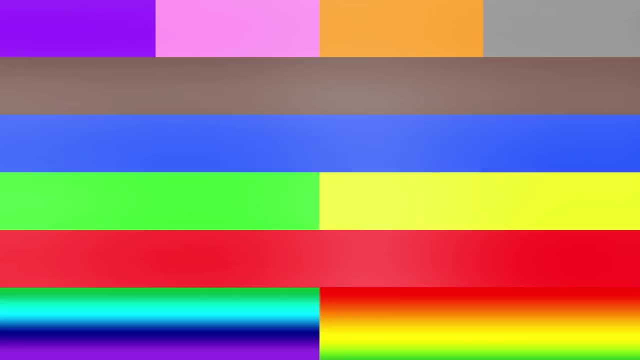 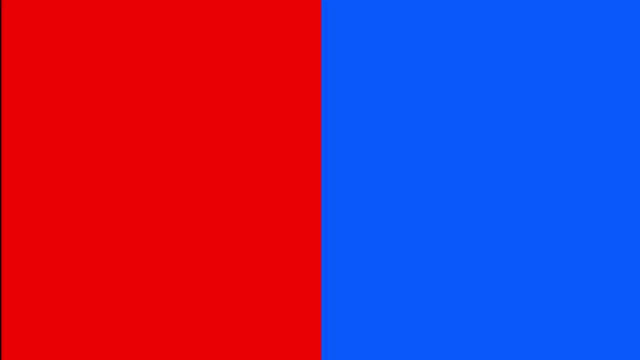 evolved to capture the true categories of color that the western languages have. I don't think Berlin and Kay have successfully proven that speakers of so-called primitive languages can't perceive the same range of colors that we can. They just use different category systems to describe them. 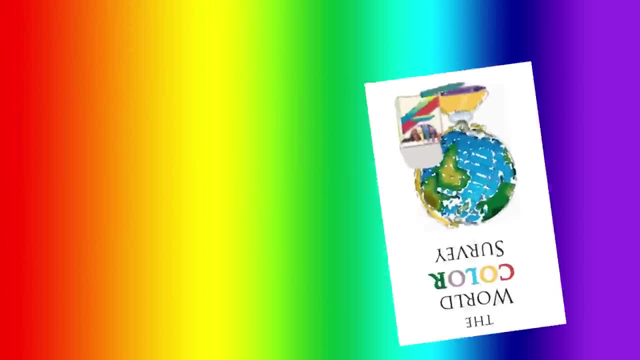 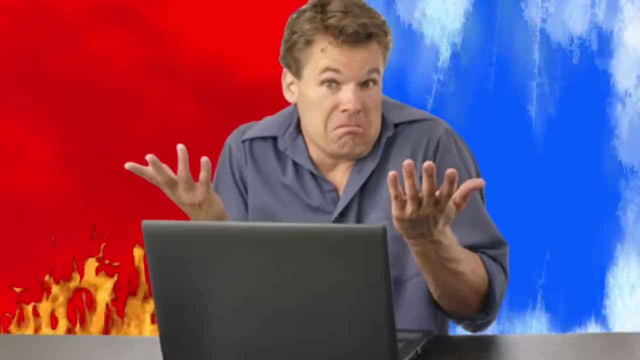 But what can be said conclusively is that, according to the World Color Survey, people all over the world seem to perceive blue as cool and red as warm. Now, this might not be particularly surprising. We make all kinds of associations between colors and concepts. 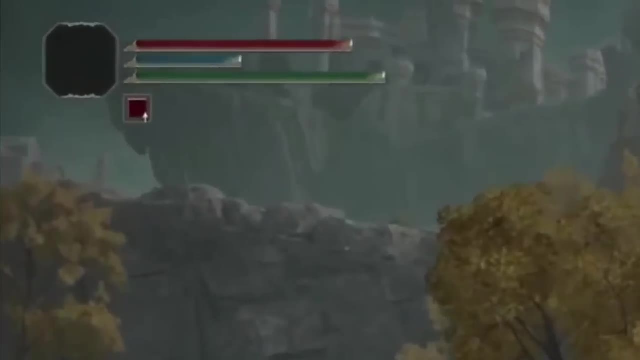 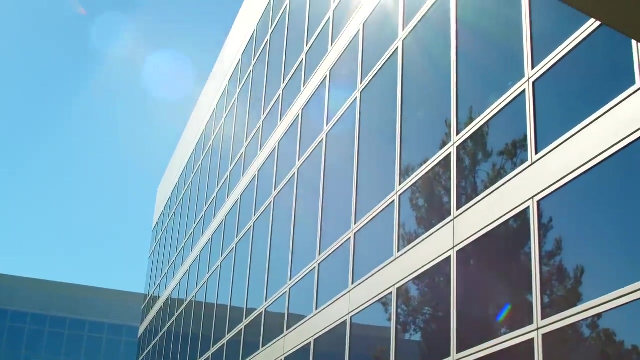 In video games the health bar is often red, the mana bar is usually blue and stamina is green. We often associate red with love, anger or power. Blue has a sophisticated, reliable corporate vibe. Orange is usually associated with energy, taste, extroversion or amusement. 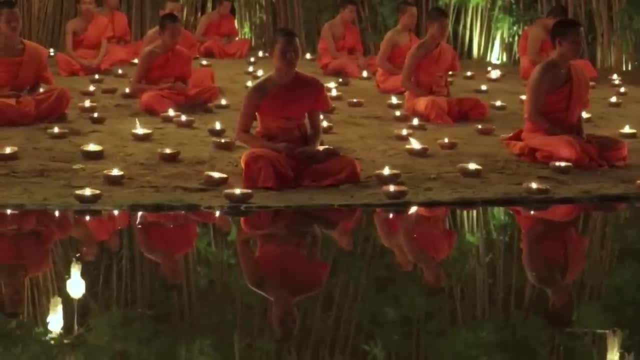 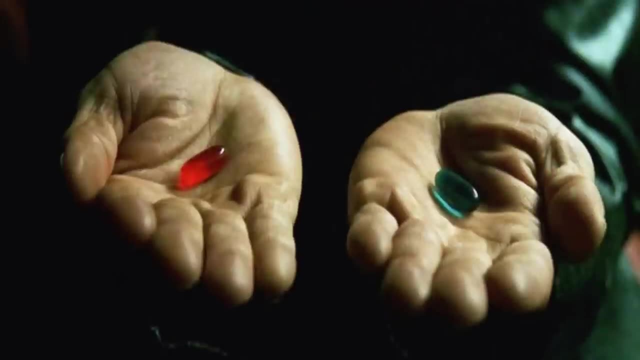 But these symbols vary cross-culturally. Buddhist monks wear orange robes, where orange symbolizes enlightenment. In placebo studies, pills with hot colors like red or yellow work better as stimulants, whereas pills with cool colors like blue or purple work better as depressants. 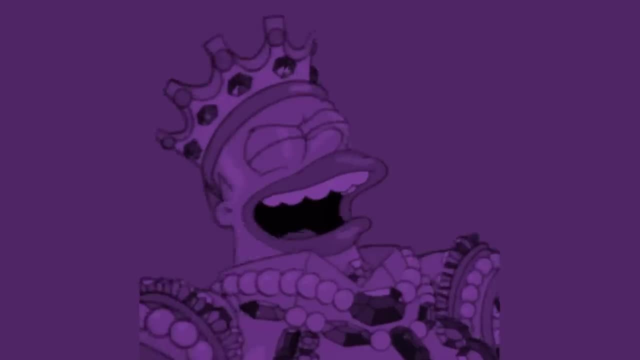 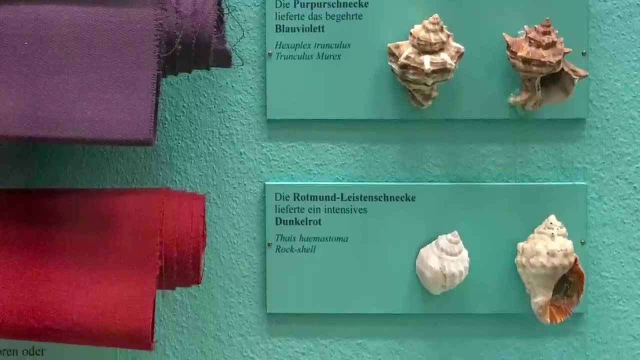 These results do seem to depend on culture, though Purple was historically associated with royalty, because purple dye was made from a species of sea snail which excreted it from a single gland, the hypobranchial gland, in very small quantities. 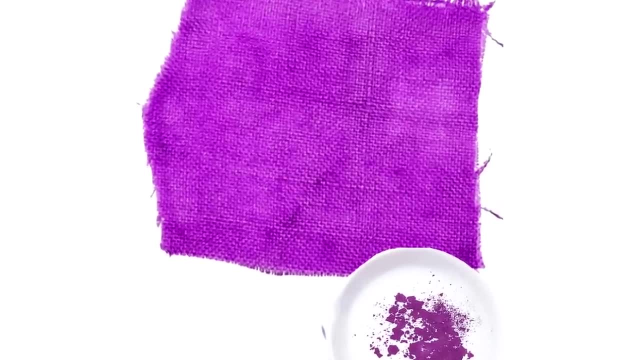 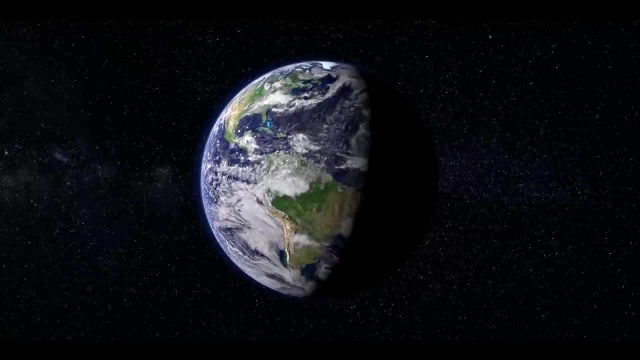 This made the dye very rare and was usually only available to the very wealthy. So just because of this coincidence that psychological association emerged. The one color association that remains consistent across cultures is cool and warm. This might just be coincidence, but it taps into a much more universal one. 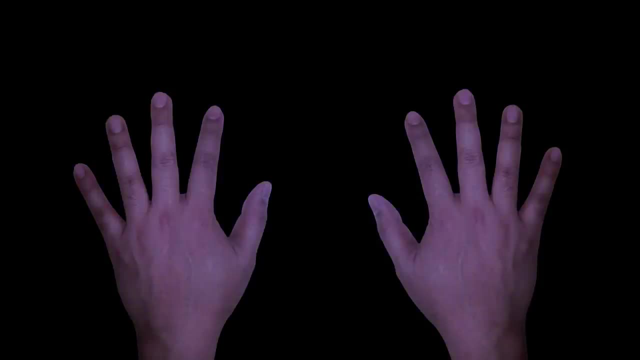 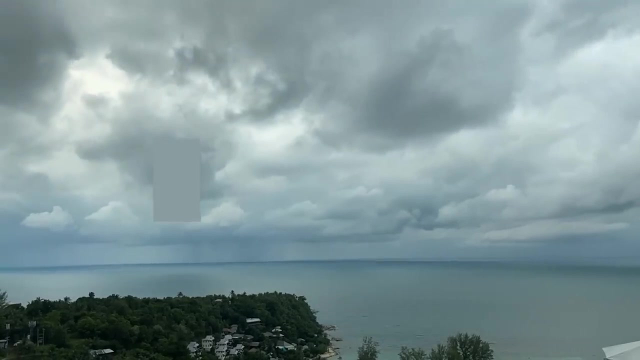 Our skin gets red when we're warm and goes blue when we're cold. When we gaze at a warm, sunny landscape, we're presented with warm colors. When we gaze at a cold, overcast day, we're presented with cool colors. 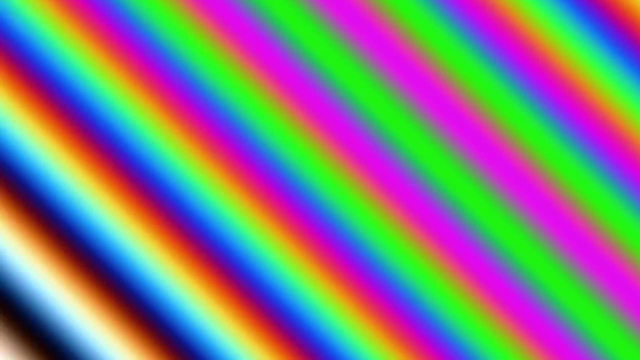 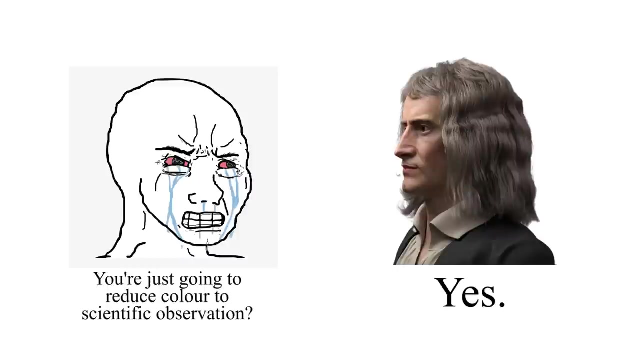 So what even is color in the first place? I'm going to argue that there are two ways of describing it, which are basically captured by two figures: Newton and Goethe. Let's start with Newton and the scientific description of light. Visible light can be understood as waves of electromagnetic radiation. 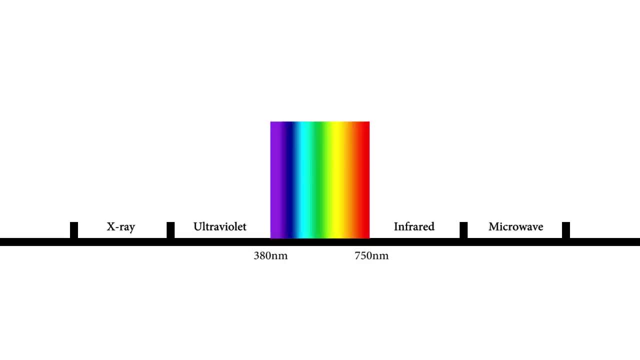 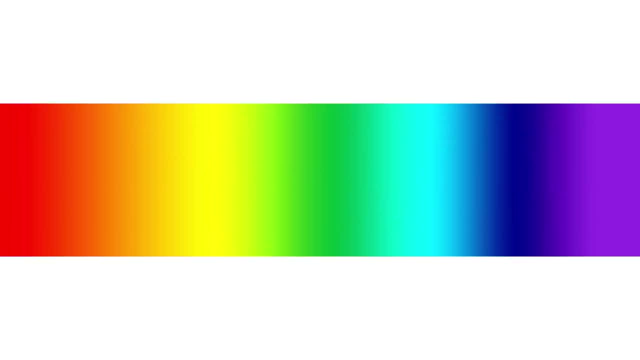 The human eye can perceive wavelengths of about the same wavelength as light. The eyes receive wavelengths of about 400-700 nanometers. One nanometer is one billionth of a meter. The visible colors on the spectrum increase from red to violet following the mnemonic Roy G Biv. 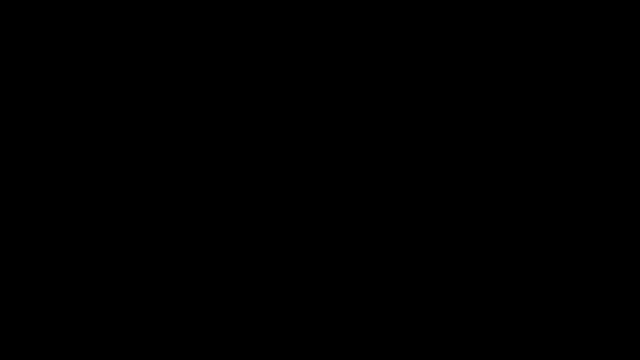 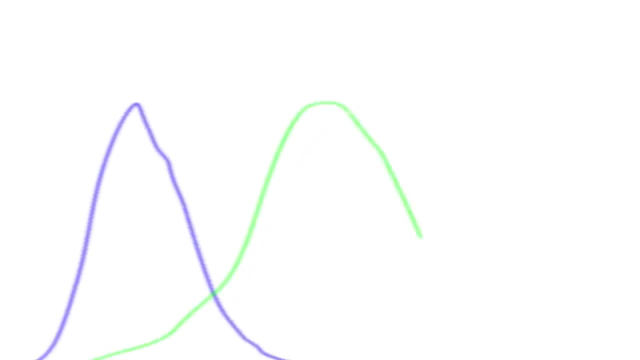 which is also a great song by Boards of Canada. The retinas of our eyes have things called cone cells. We have three types of those. One responds really well to blue light, one to green and one to red. The colors we see in the world are the result of the way in which these receptors respond. 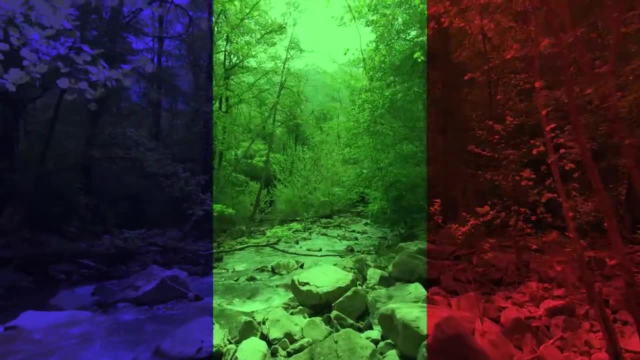 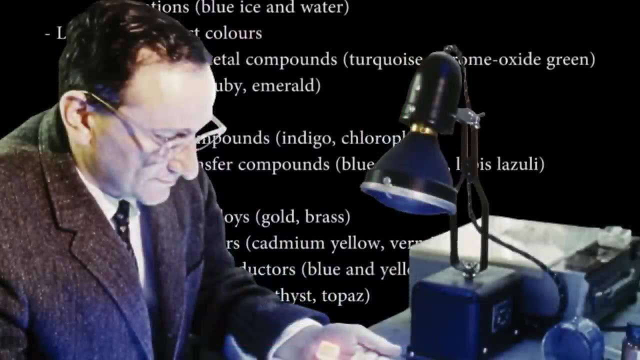 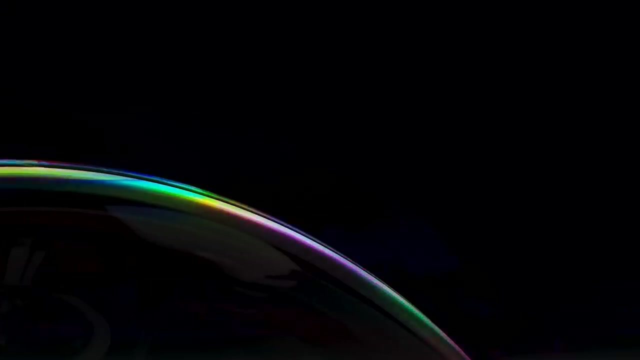 to different levels of blues, greens and reds are reflected by materials. In the book The Physics and Chemistry of Color by Kurt Nassau, he enumerates 15 different causes of color, including everything from the incandescence of flames, the rotations of blue ice and water and the interference of soap bubbles. A lot of. 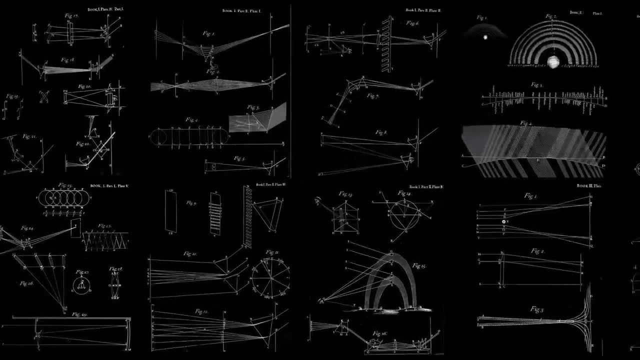 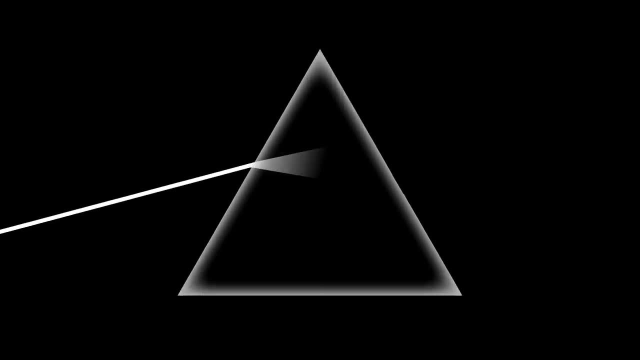 our scientific understanding of color has its roots in an experiment by Isaac Newton conducted in 1704.. He constructed a triangular prism and shone a sunbeam through it, refracting its light. Colors emerged from this process of refraction, which he called a spectrum. 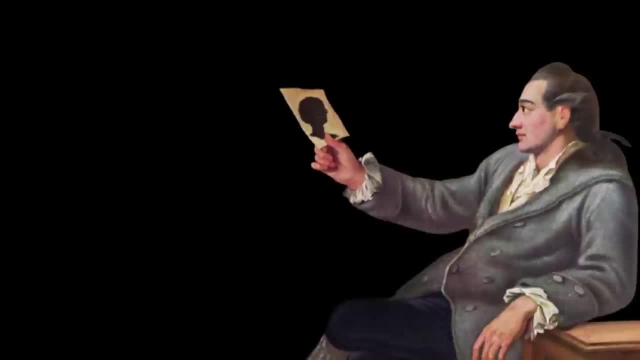 About a hundred years later, Goethe, the German poet responsible for Faust, became interested in color too. Goethe knew about Newton's experiments and tested it himself with prisms he borrowed from a friend. As you do, We've all got that one friend who always has a bunch of prisms on hand. 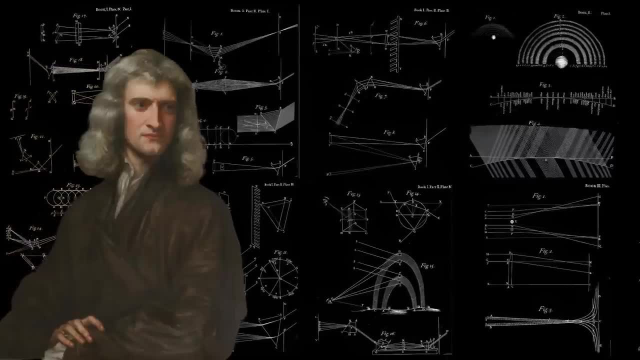 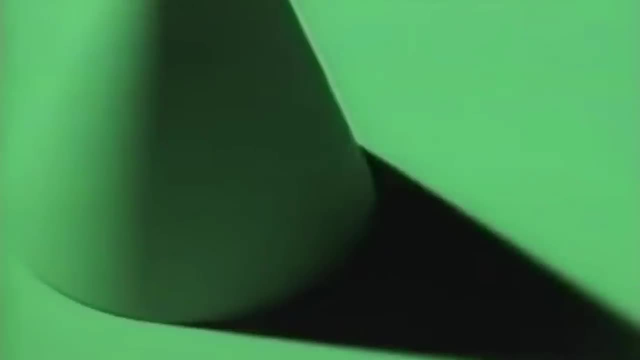 While Newton was concerned with systematically analyzing color in a scientific way, Goethe was interested in color as we see it. He conducted experiments with colored shadows. He noticed that through color he would be able to see what color was if a colored light is shone on an object and a white light is shone on its opposite side. 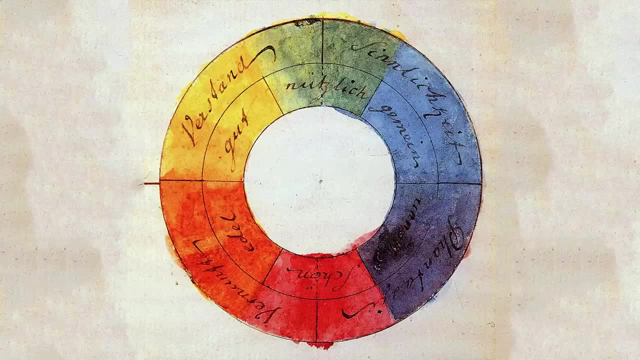 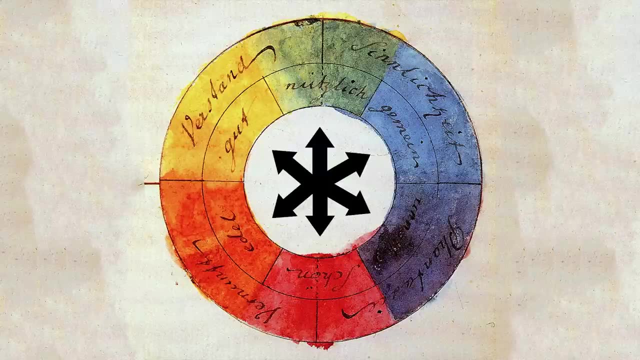 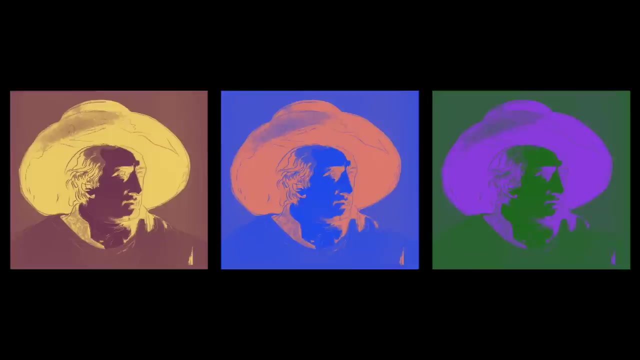 we perceive the shadow as the color's complement. In his color wheel, he situated these complementary colors opposite one another In his view. our perception strives for unity: Yellow demands violet, orange demands blue, purple demands green and vice versa. Another instance of this is the 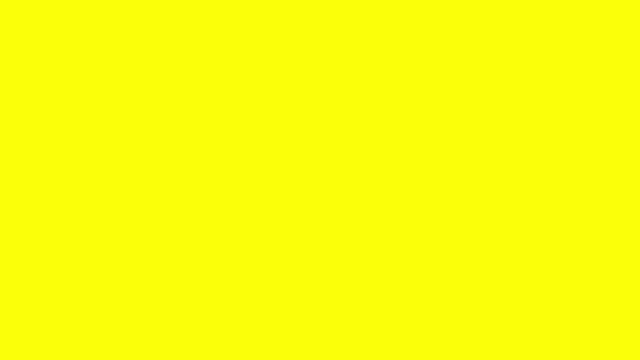 phenomenon of accidental color. Here I've made the screen yellow, Pause the video and stare into the yellow for 30 seconds or so and then unpause. Your eyes had become accustomed to the yellow and when the screen abruptly switched to white, your perception conjured a violet hue. 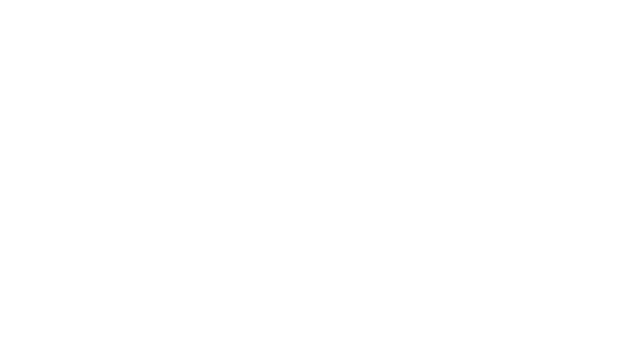 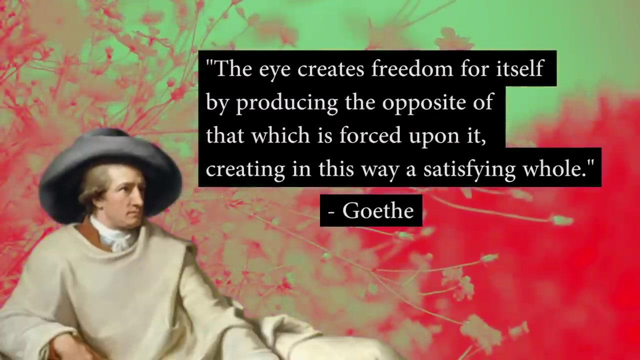 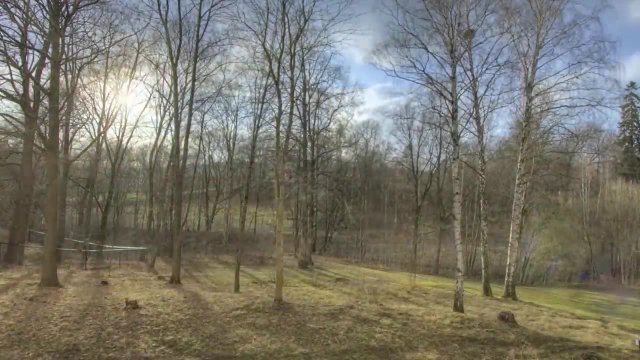 Our eye wants to bring harmony to our visual experience. The eye creates freedom for itself by producing the opposite of that which is forced upon it, creating in this way a satisfying whole. Goethe was also very concerned with how color affects us. The color palette of a scene tells us about the seasons and cycles of our world. 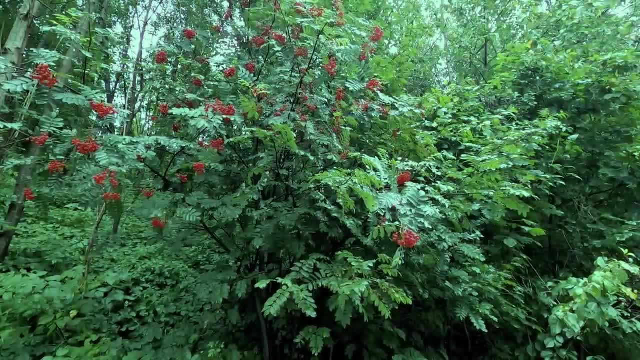 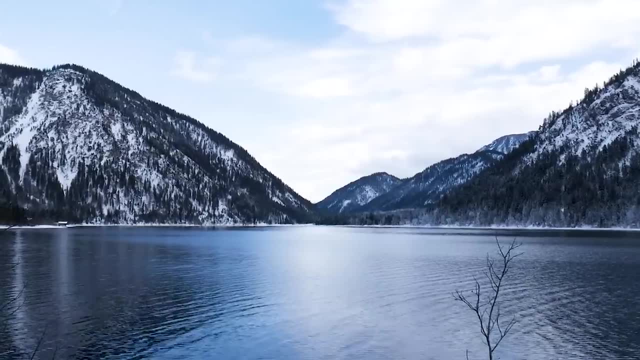 They show us how to tell one thing from another. We wouldn't be able to spot these berries if they weren't brightly colored. We see certain colors as warm and textural. We see others as cold and spatial. Yellows seem to come towards us and blues seem to recede away. Not only is color associated. 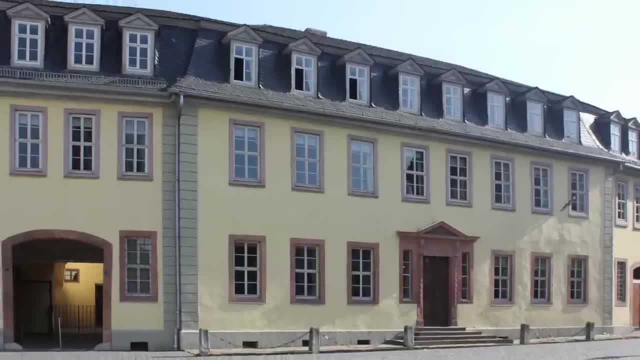 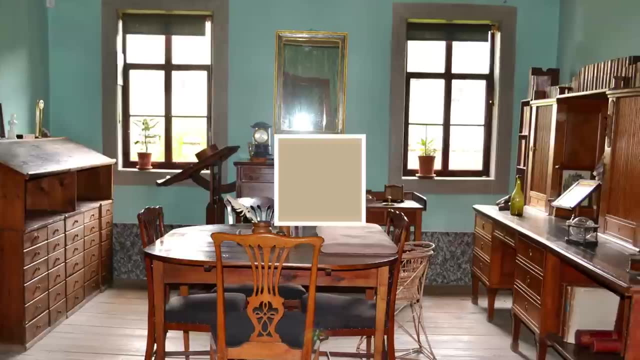 with temperature, but also proximity and distance. Goethe took this so seriously that his home was painted very deliberately with a yellow dining room to create a sense of warmth and pleasure and a greenish-blue study to promote a stimulus. The red color in the sky is the dark and the blue will create a sense of warmth and pleasure. 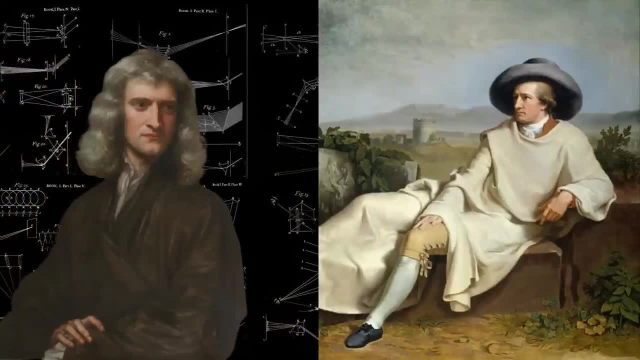 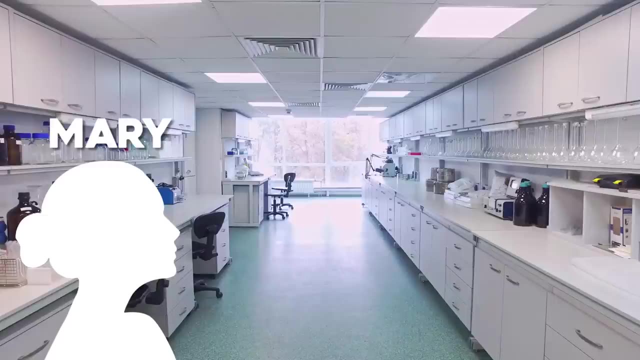 So it's hard to get up in a place with a sunny sky. In a way, you can see a unique and stimulating, calming environment. Where Newton's approach was analytic, Goethe's approach was poetic. These aren't necessarily contradictory views either. They're just two ways of looking at things. 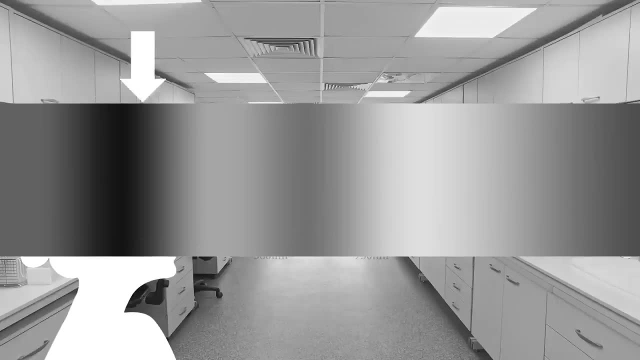 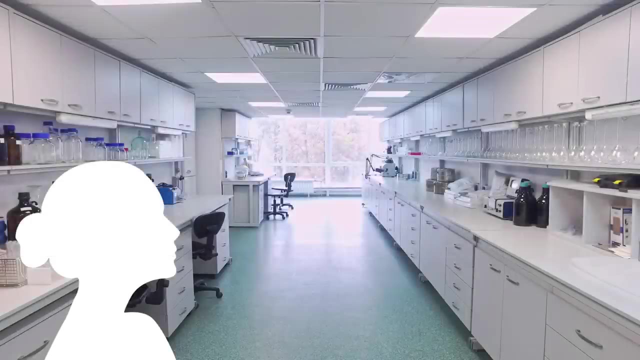 To elucidate this distinction, consider the scientist Mary. She exists in a black and white world, But she can still study color. She has access to physical descriptions of color. She can tell you which wavelengths correspond to each color. take in the perceptual experience of color for the first time. The question is: will Mary gain any? 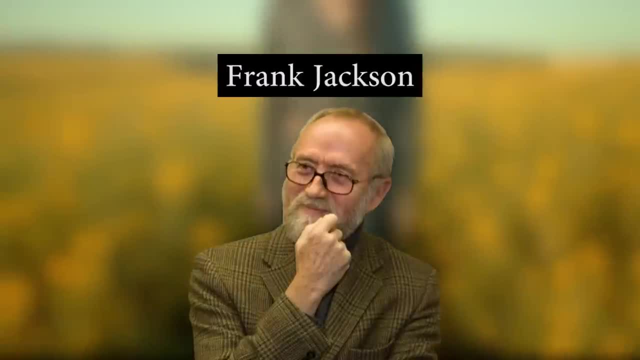 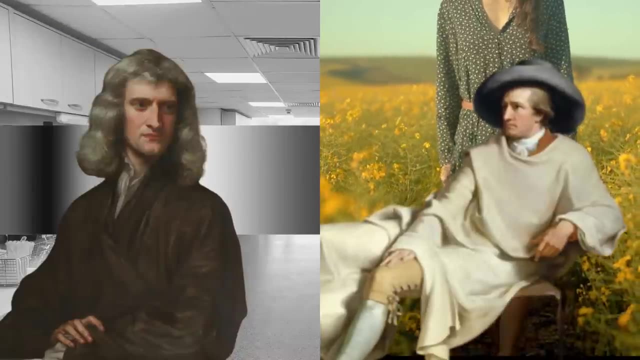 new understanding. This thought experiment was proposed by Frank Jackson in 1982.. Newton approached color as Mary did from her black and white world, while Goethe was concerned with the understanding Mary achieved from actually seeing color. Goethe urged that physical descriptions of color only. 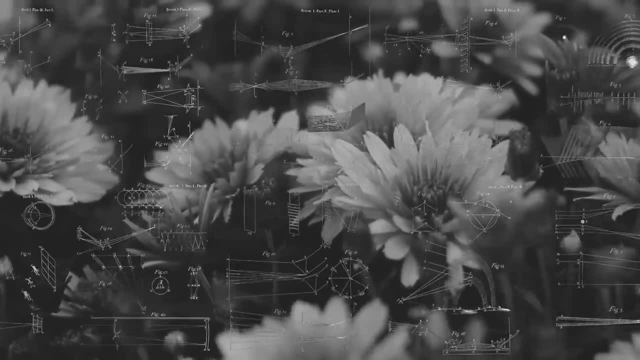 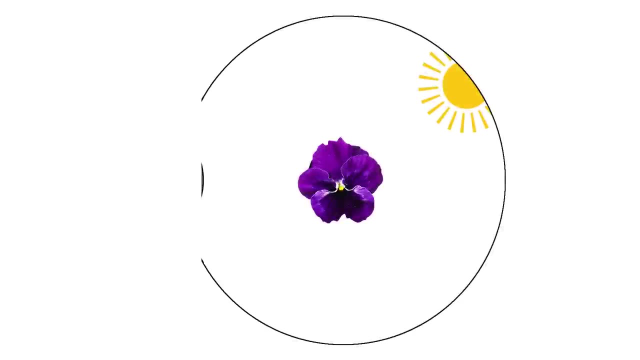 tell half the story. We can't separate the color in the world from the color as we see it. He didn't view humans as passive observers of things. For him, the outer world calls forth the inner world meeting in a participatory interaction. Color isn't just light particles out there in the world. 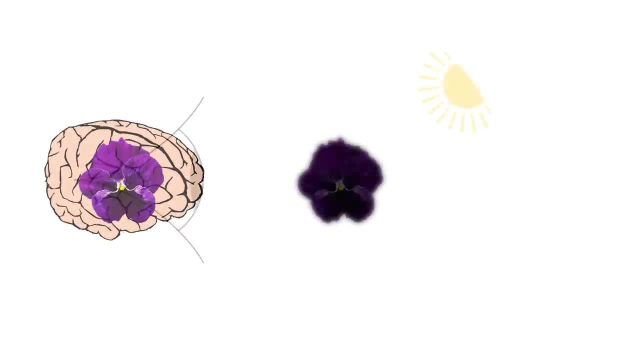 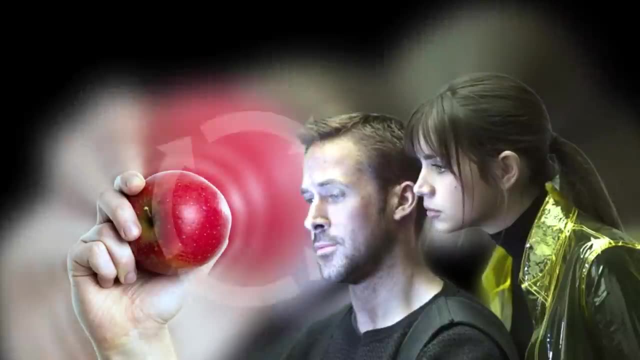 nor is it a conscious representation of the light in the world. Instead, color arises through the interplay of light and sight. So in this way, we don't just take color in. Color emerges from our interaction with the world. In a sense, we put a little bit of 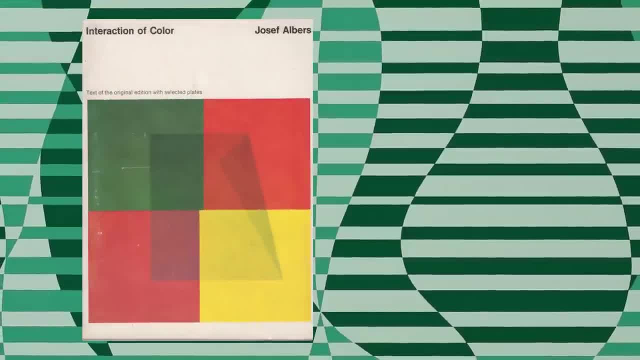 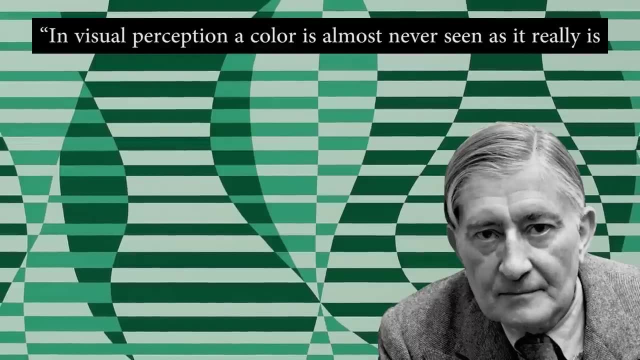 ourselves into the color. In the book Interaction of Color, the artist James Goethe wrote. Joseph Albers discusses the way in which color is relative. In visual perception, a color is almost never seen as it really is, as it physically is. This fact makes color the most relative. 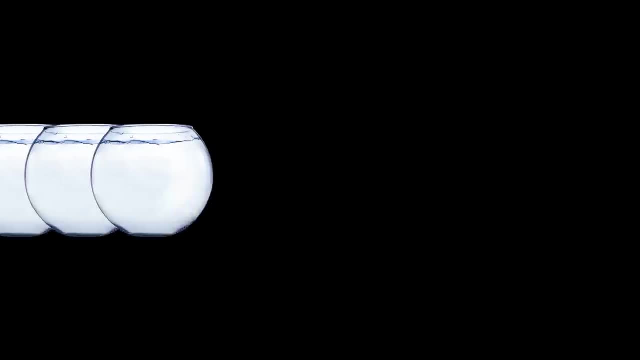 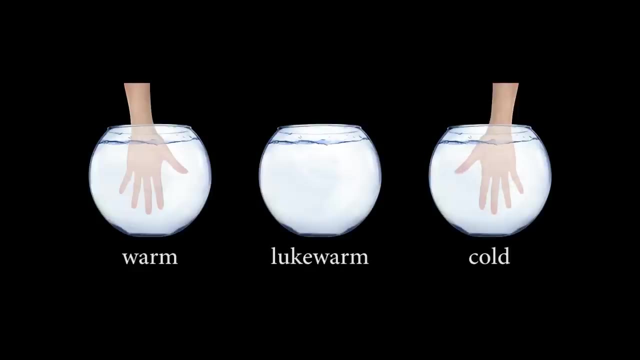 medium in art. Here's an experiment he describes. There are three pots of water in front of you containing warm, lukewarm and cold water. You dip your hands into each outer container- left hand in the leftmost pot and right hand in the rightmost pot- You perceive two different. 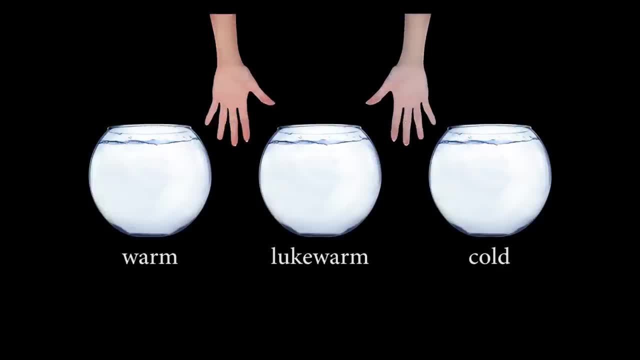 temperatures: warm on the left and cold on the right. But then you dip both hands in the middle container, You perceive two different temperatures again, but this time in reverse order: Your left hand feels cold and your right hand feels warm, But in reality the water is neither of these. 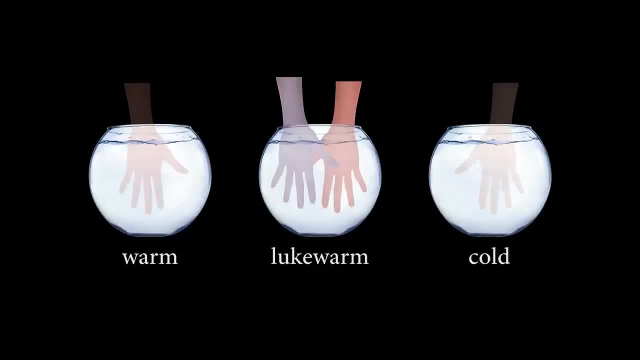 temperatures: It's lukewarm. The context of our prior experience altered our perception, In the same way that the relative temperature of our hands deceives us in this haptic illusion where physical fact and our conscious experience don't match, optical illusions also deceive. 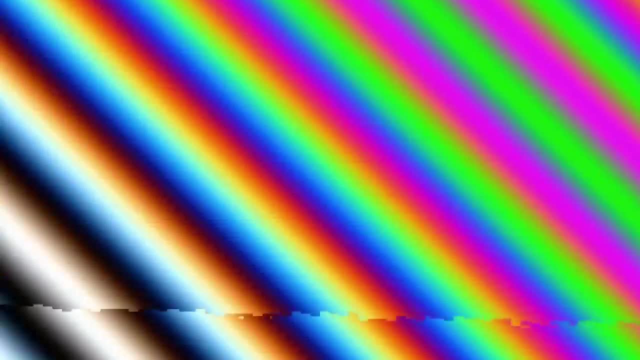 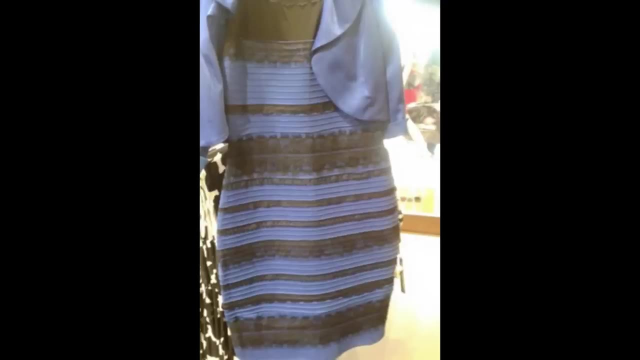 They cause us to see colors other than those with which we are confronted physically. Remember this dress As of the recording of this video. this meme blew up just over 8 years ago. People argued endlessly over whether the dress was black and blue, or white, and 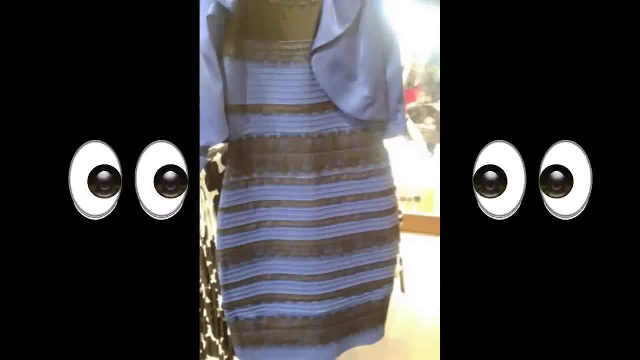 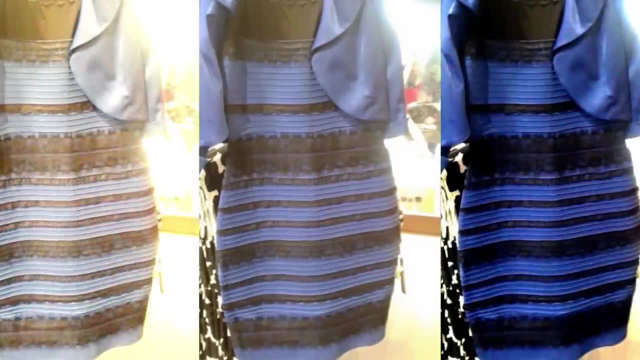 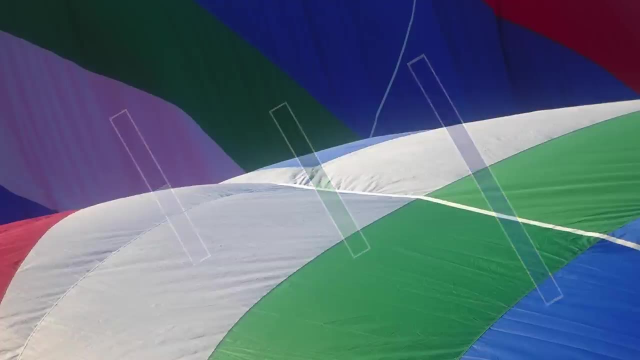 gold. The reason nobody could agree was because people's visual systems were interpreting the photograph in different ways. In particular, different people assumed different conditions of illumination. When we look at a scene with different levels of illumination, we're able to recognize different colors as the same- A phenomenon called color. 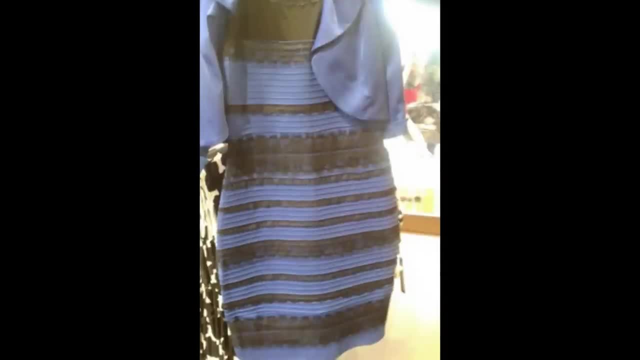 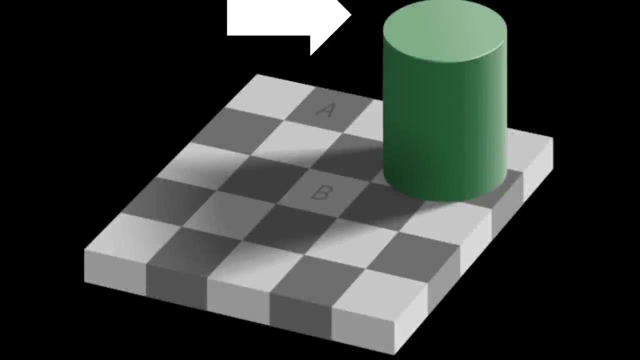 constancy. Depending on how you initially interpreted the illumination of this photograph, you could see the dress with completely different colors. Here's another illusion you've probably seen before. We have a cylinder casting a shadow on a floor of tiles. It appears that the tiles A and B are different colors. A looks gray while B looks 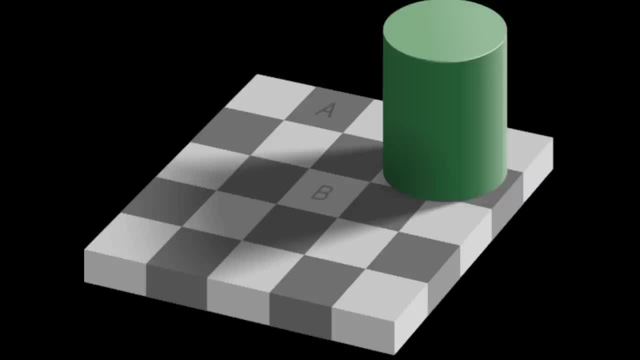 white, But when you scrutinize the image more closely, you realize that these tiles are in fact identical. The context of the scene and the interpretation we have for what's happening is changing the way we see these colors. We're able to see the image in a different way. 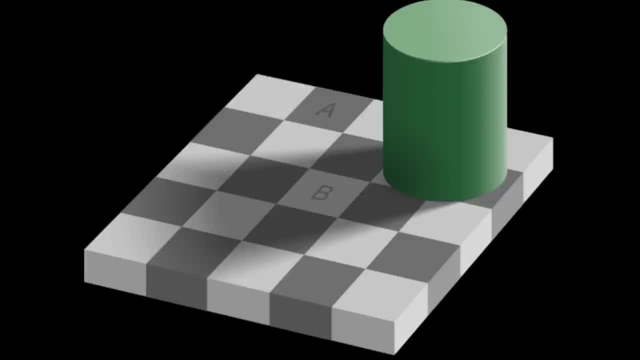 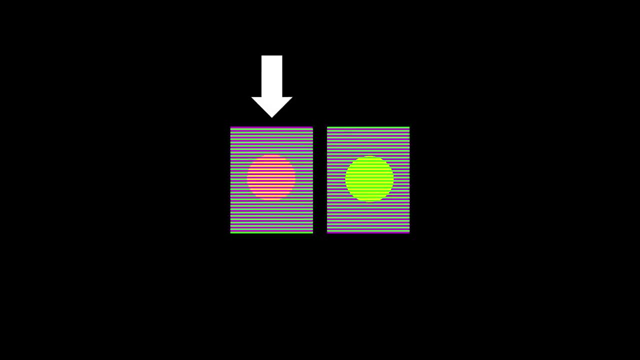 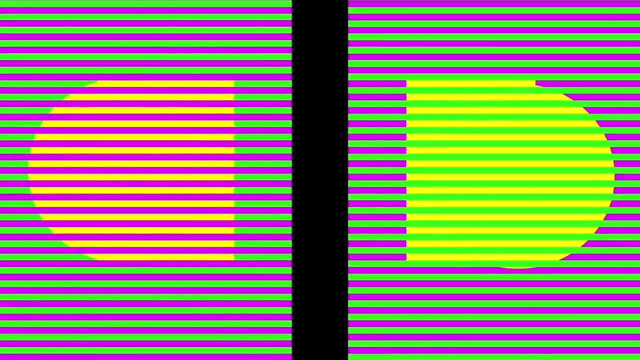 Okay, last one. Take a look at the circles in the middle. The left circle appears red and the right circle appears green, But once again, if I zoom in, it becomes clear that each circle is in fact yellow. All of these illusions demonstrate: 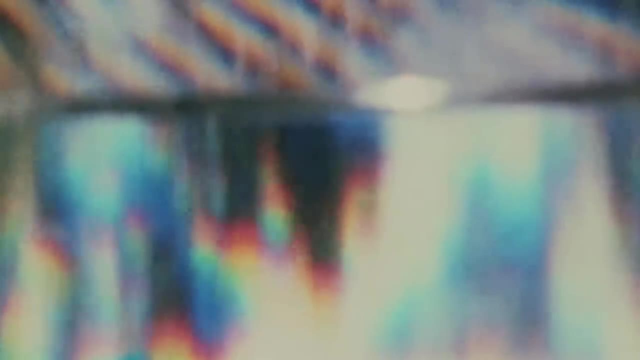 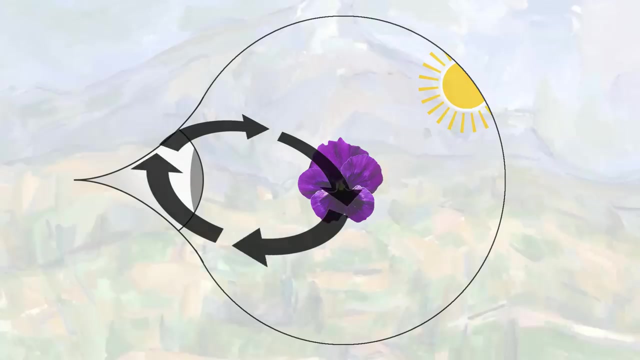 a key insight that Goethe knew. Colors, as we see them, are not merely light. Color is a conscious event resulting from the interplay between the observer and the observed. The French post-impressionist artist Paul Cézanne wrote that color is. 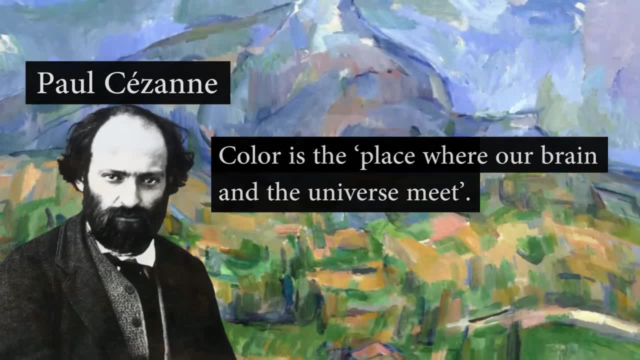 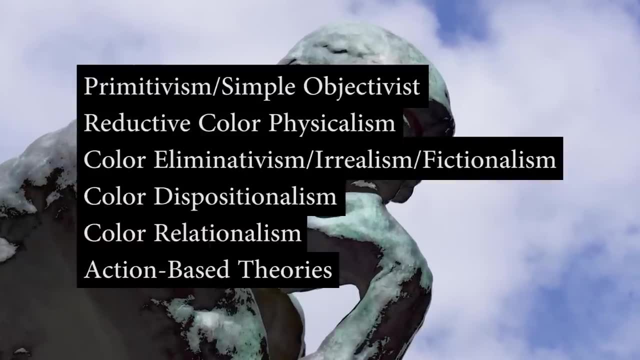 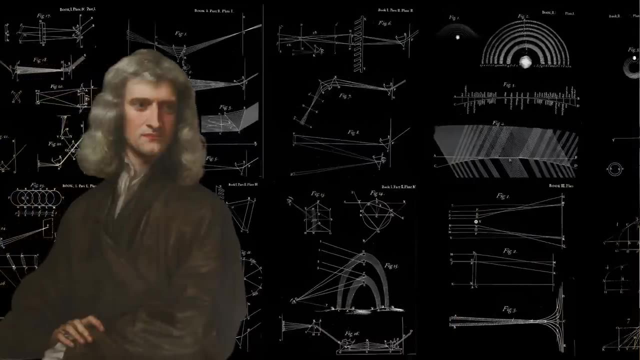 the place where our brain and the universe meet. So what do philosophers make of all this? Well, there's a number of different takes people have, but in this video I'll be discussing two theories that I think capture the ancient disagreement between Newton and Goethe. Let's start with the Newton side of things, and one of the most famous. 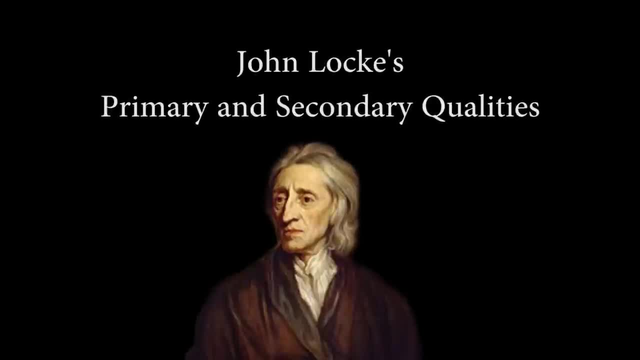 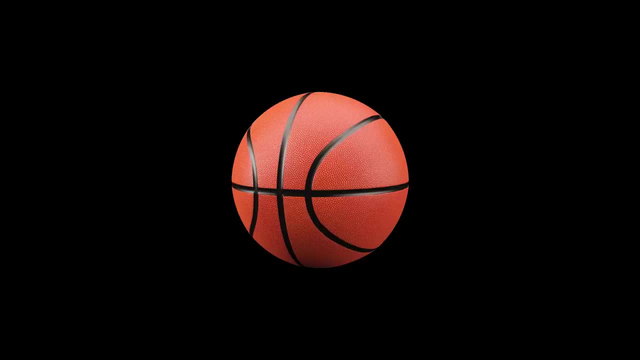 properties of things as they are in the world, independent of our perception. Take a basketball, for example. The fact that the basketball is spherical is an inherent property of that object and does not depend on an observer seeing it that way. Then there are secondary qualities. 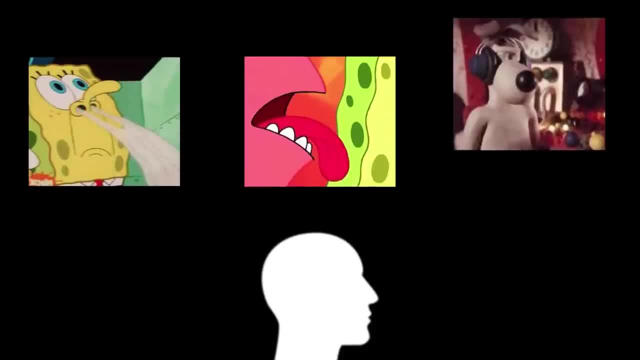 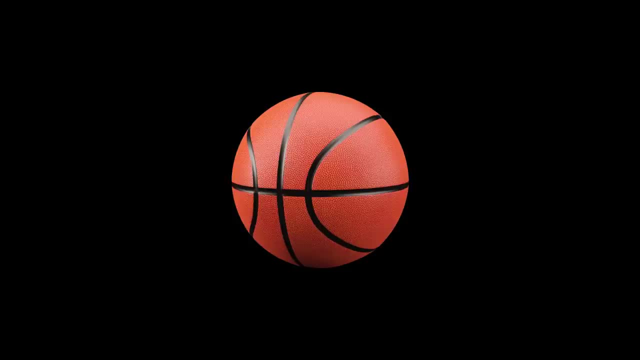 the stuff that depends on the observer, like smell, taste, sound and, of course, color- The basketball being orange and the sound it makes when you bounce it- are each secondary qualities. Objects don't exactly have colors in this way, but they have dispositional properties. 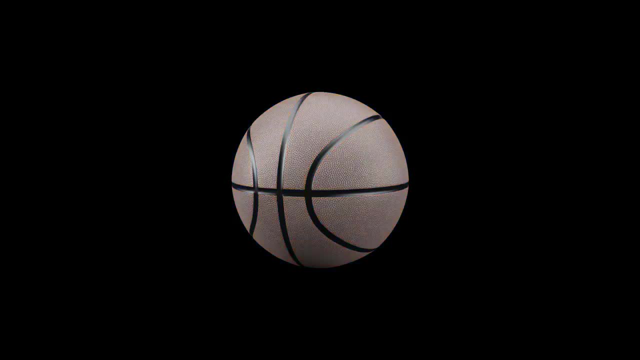 to give rise to colors. The basketball is not orange itself, but exists in such a way that it appears orange to an observer when they look at it under the right conditions. Some people call this a received view of color, since the properties of the object 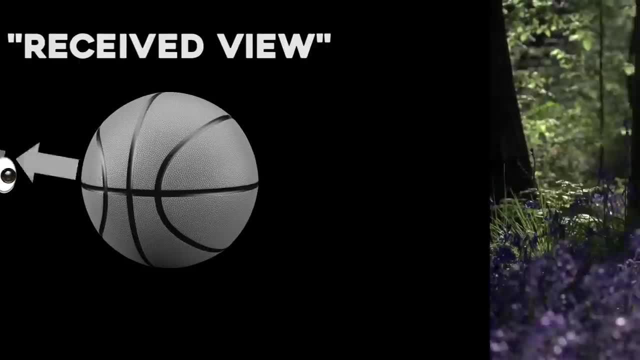 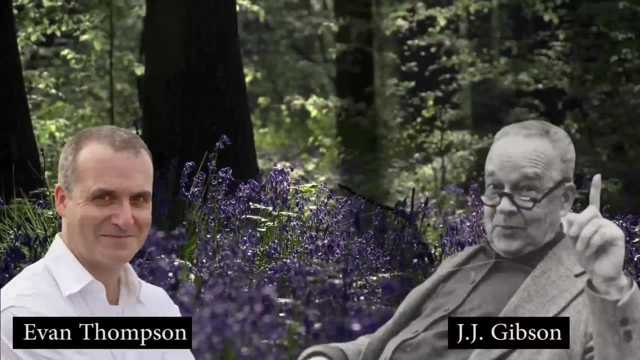 result in the observer receiving that sense experience. On the other side of things, we have a take that's more in the spirit of Goethe. Evan Thomson, JJ Gibson and some others put forward what's known as an action-based ecological theory of color. On first glance it 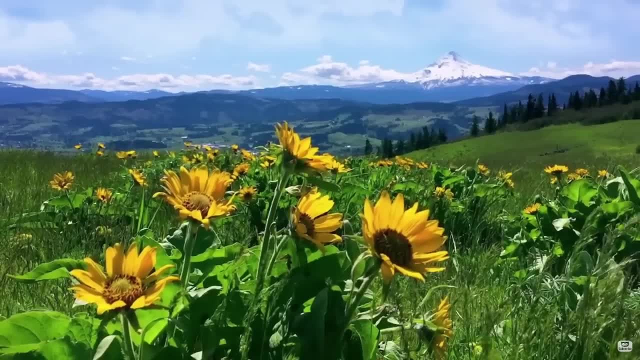 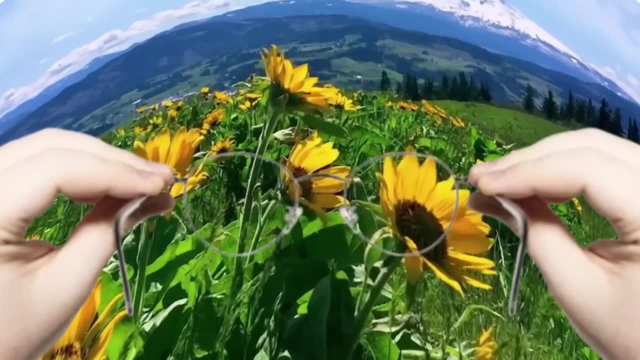 seems pretty similar to the received view. They still don't consider color's intrinsic properties of things in the world. independent of any perceiver. It depends in part on the perception of the color itself. Color is a relational property connecting the environment with 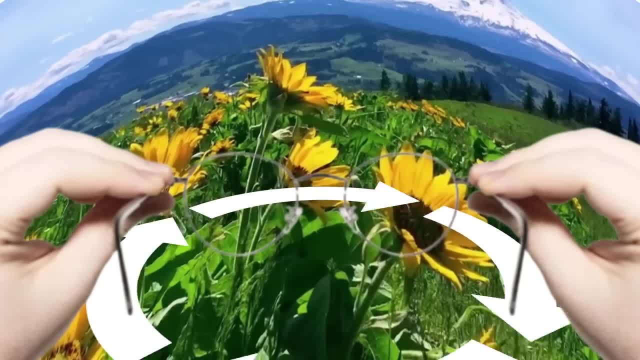 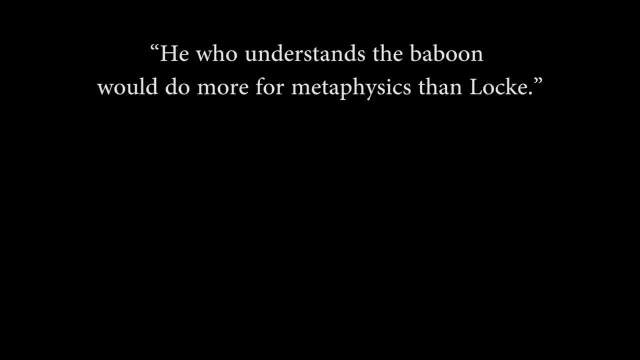 the perceiving animal. But this view also wants to emphasize the fact that at the end of the day, we're still basically animals. He who understands the baboon would do more for metaphysics than Locke. That quote is from none other than Charles Darwin. Biologists will always tell. 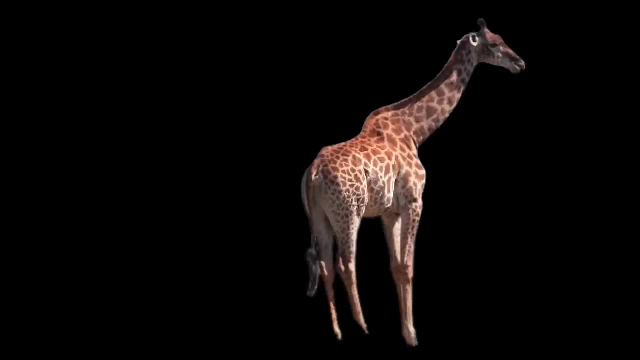 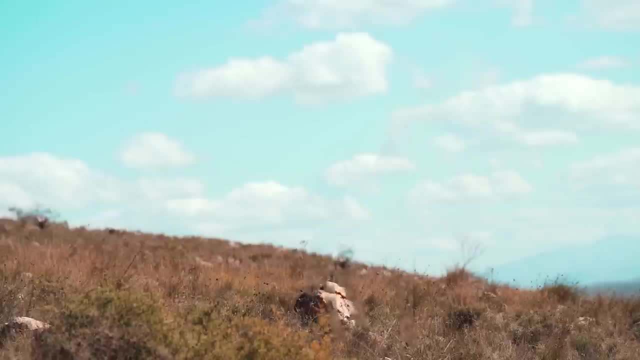 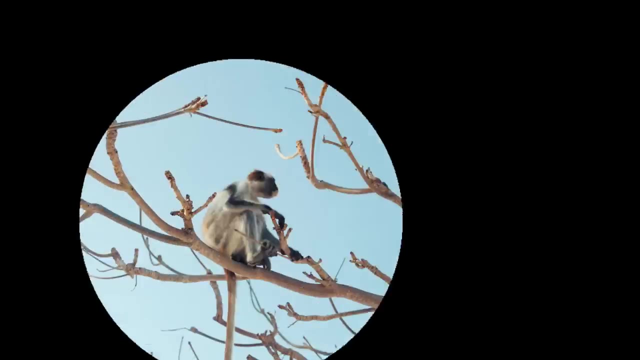 organism's environment, or niche, can't be understood apart from the organism. in fact, the animal and its environment are connected in a much deeper way than you might expect. an organism finds itself in an environment, but they don't just hang out there. they interact with their surroundings based on the 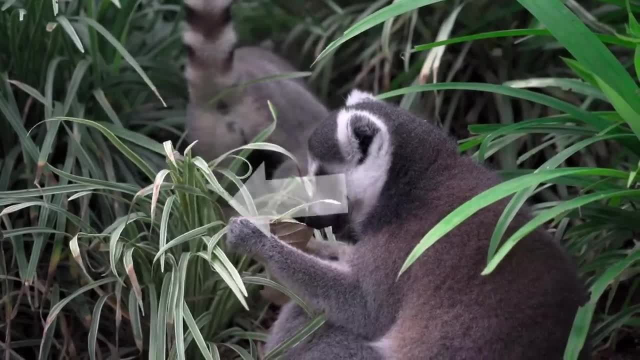 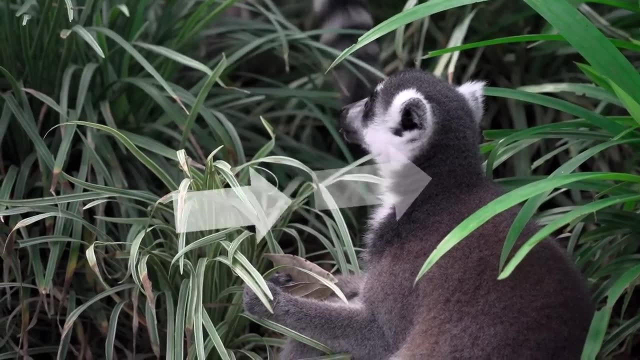 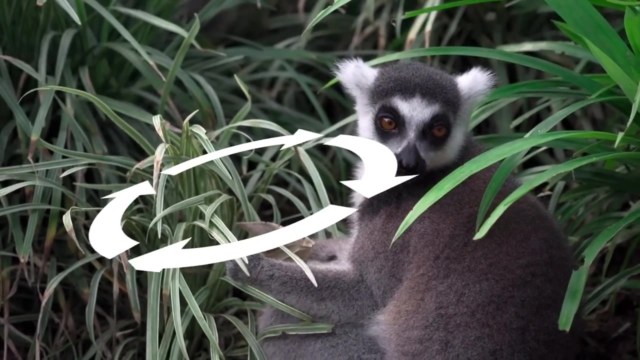 physical signals the environment gives them. through this, they transform the environment and simultaneously the environment itself transforms the organism by defining what traits are selected. evolutionarily, The organism and the environment co-determine each other. This co-determinacy is a bit of a problem for people like Locke and Newton. 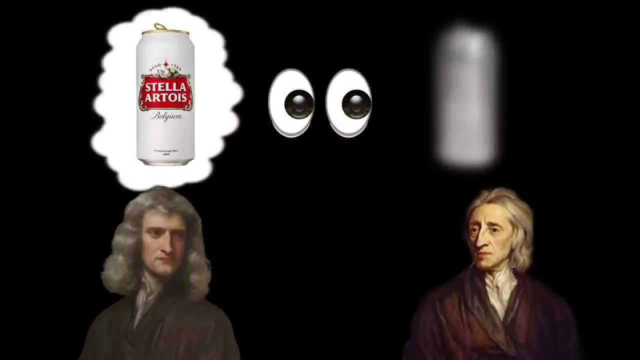 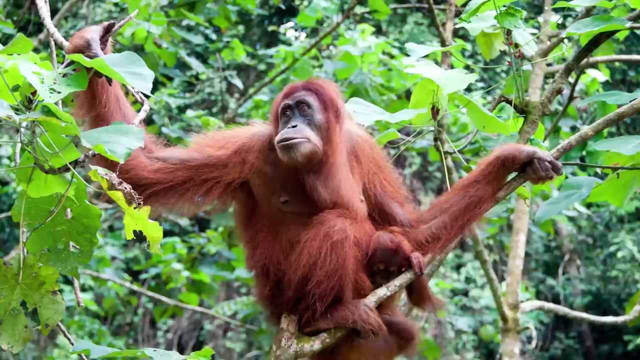 For them, perception involves representing items of sense, data, which are the immediate objects of perception. These representations stand in for some physical object in the external world, So we aren't actually looking out at the world, We're looking through our representations. This view treats the animal and its environment as separate systems. 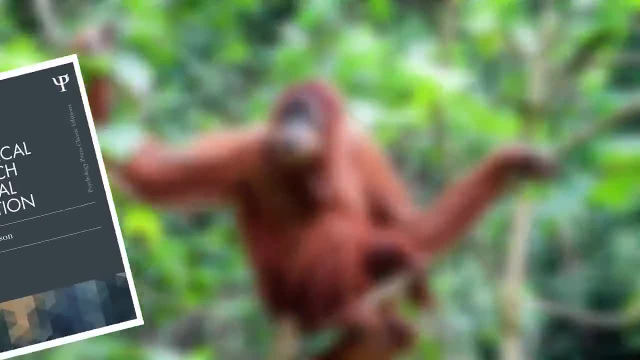 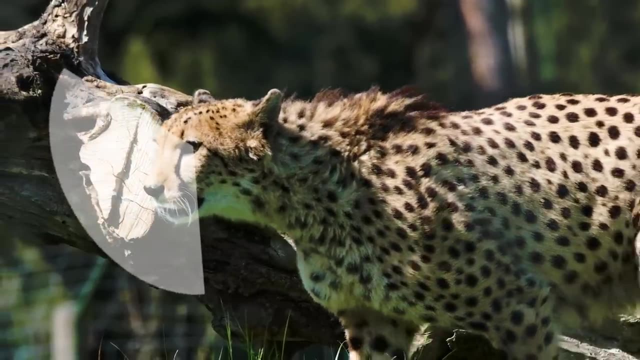 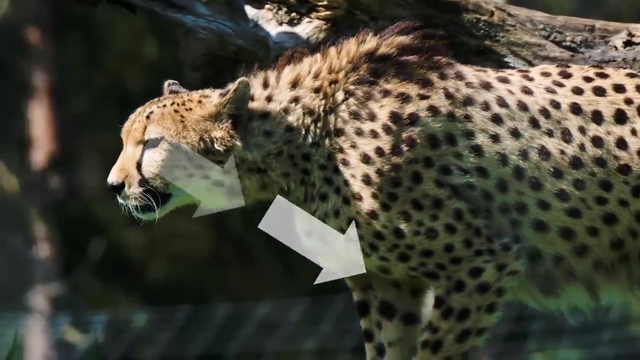 rather than two components of one system. In the ecological approach to visual perception, Gibson expresses some issues with this. take As animals. our perception is always guided. Perception and action evolve together and are inseparable. Our perception guides the activity in our motor system. 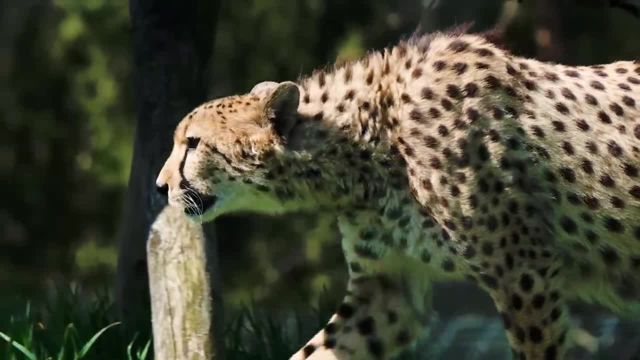 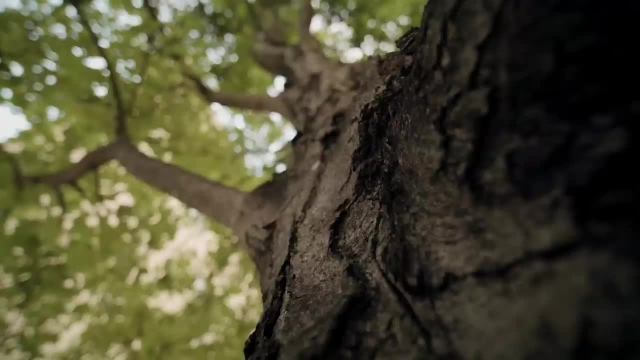 and our motor system guides perception. For Gibson, environments have particular relational properties called affordances, things that give us an opportunity to interact with them. Trees, in relation to certain animals, afford climbing. They can be described as climb-up-able. 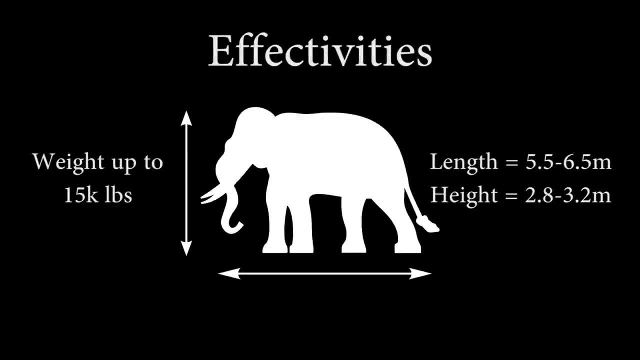 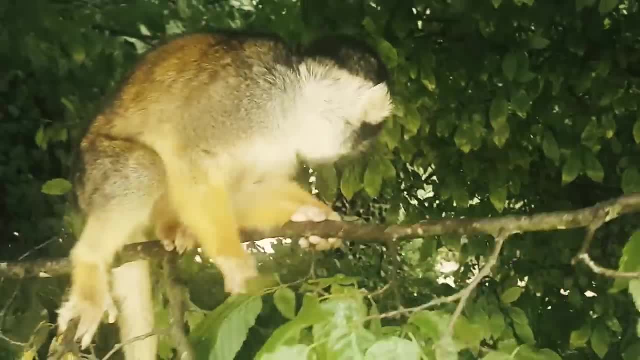 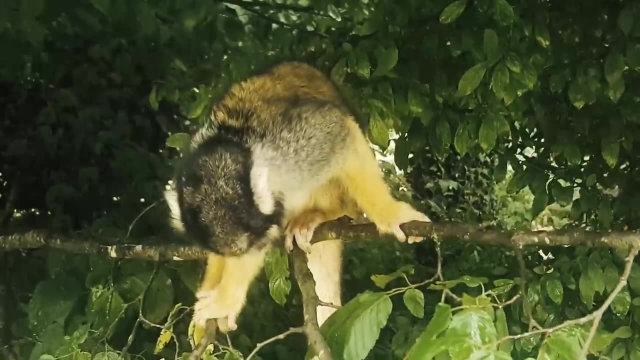 The other side of the coin is effectivities, the properties of animals that allow an opportunity for interaction with the environment. Lizards and monkeys can climb things, so they possess the effectivity climbing thing. These kinds of properties are really weird, since they're almost objective and subjective at the same time. 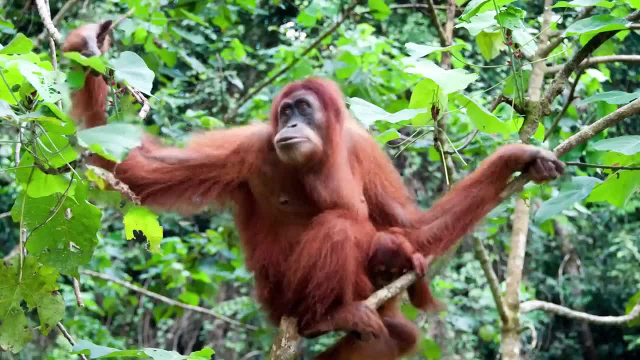 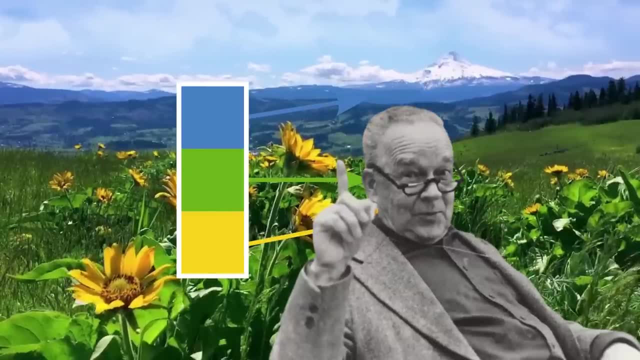 It's both a fact of the environment and a fact of behavior. It's both physical and psychological. Gibson ultimately wants to say that the colors we see have lawful correlations with particular ecological properties like affordances. So what's even the difference here with the Lockean or the Newtonian view? 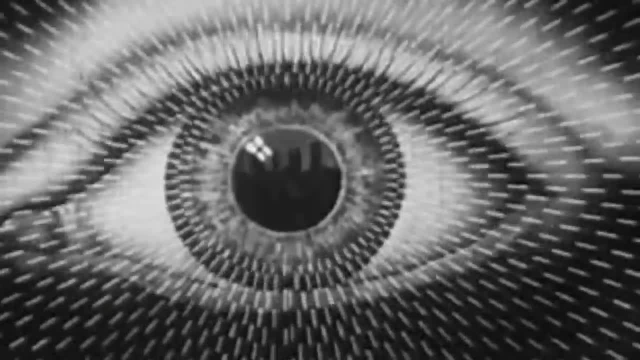 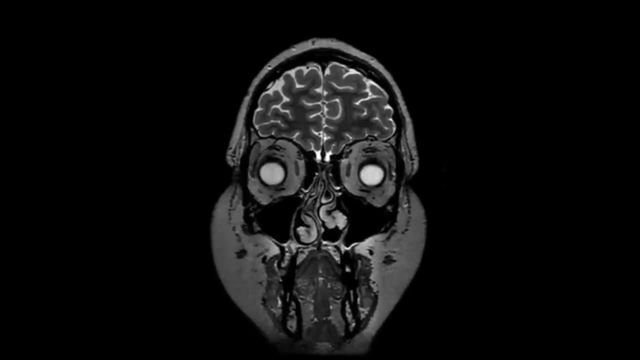 They both agree that color depends on the observer and can't be understood as intrinsic properties of the world independent of our perception. Neuroscience can model the features of color as we perceive them, so it might be tempting to conclude that object color is really just an illusion. 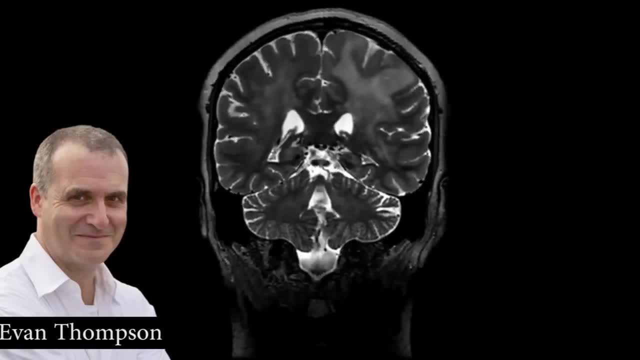 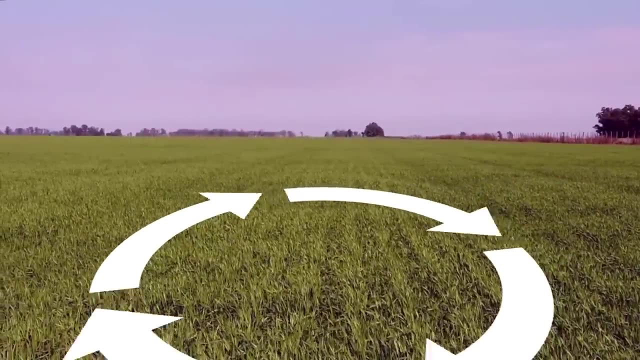 and we can reduce it to neural states in the visual system. But Thompson and Gibson want to avoid this. Instead of situating color exclusively in the brain, they want to take into account the relation with the environment Instead of color being a dispositional property on the physical level. 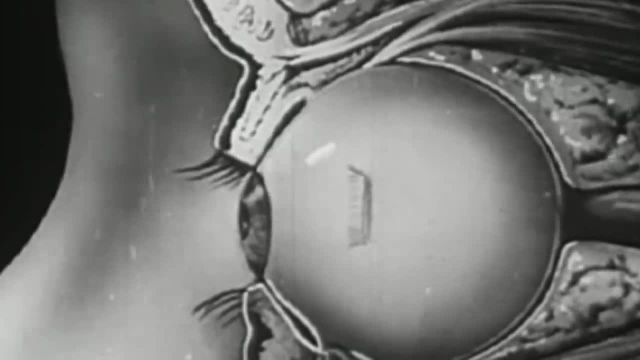 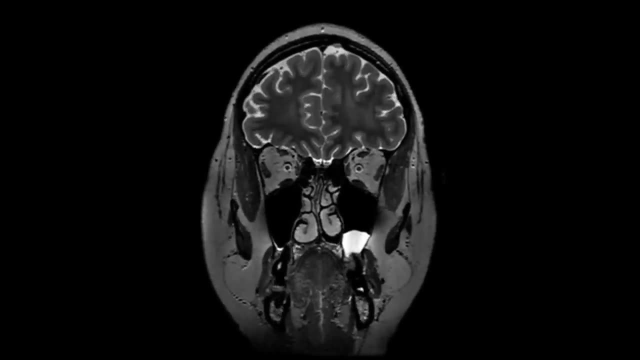 it's on the ecological level. This view is naturalistic in that it strives to be in harmony with visual science, But that doesn't mean it wants to reduce animals like humans to collections of neural activity and physical processes. The perceiver is treated as an active, exploring animal. 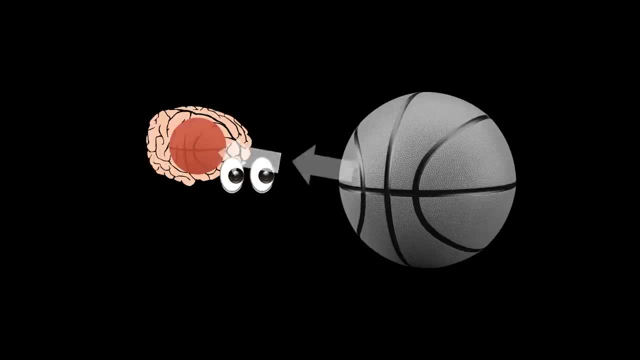 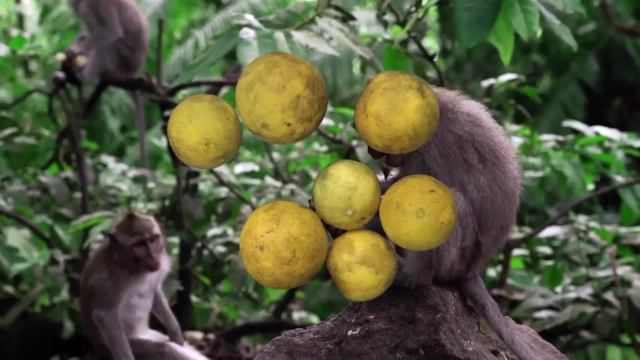 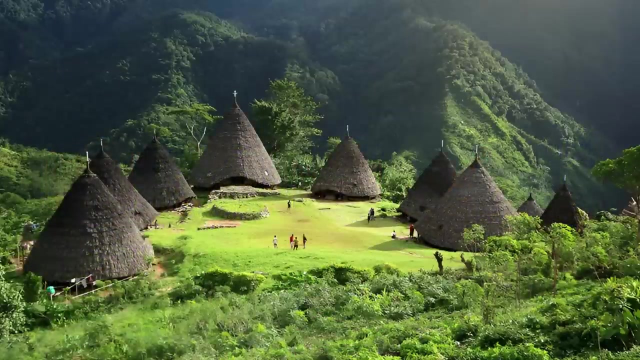 rather than a disembodied spectator who just takes the colors in. Colors are connected with affordances and effectivities, especially in their roles as categories and signals to us to satisfy our adaptive ecological needs. They reveal what the environment can do to us and what we can do to the environment. 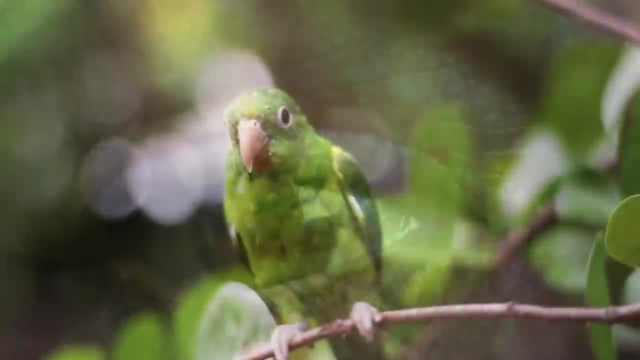 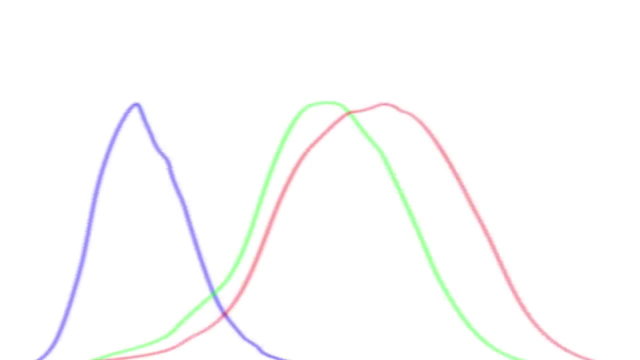 It's also worth noting that the colors we see are not the same colors that other animals see. I mentioned earlier that humans have three types of cone cells in the eye that process color, which makes us trichromats. But this is not the norm. 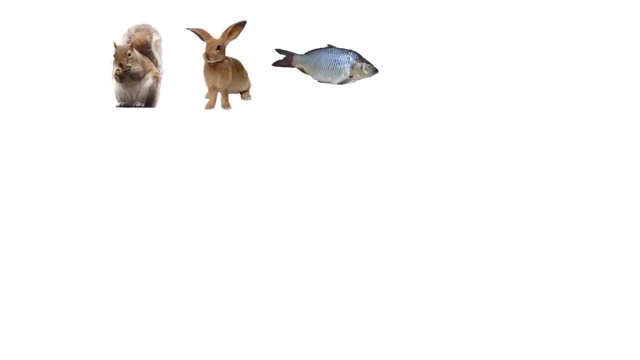 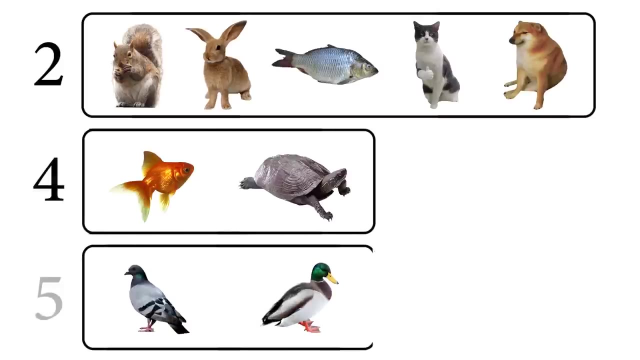 Animals like squirrels, rabbits, some species of fish and possibly cats and dogs only have two. Goldfish and turtles have four, and pigeons and ducks might even have five. Even within these categories there's variation. Humans and honeybees are both trichromats. 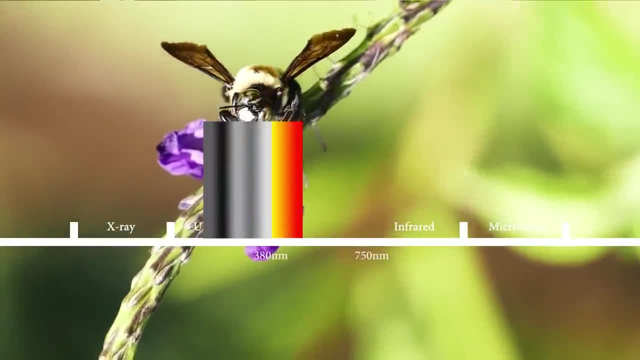 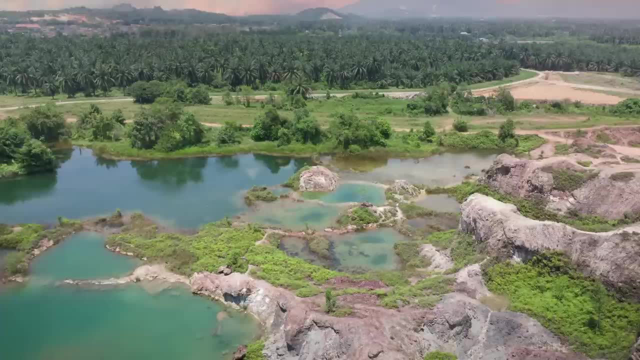 but the colors. the honeybee sees is shifted towards the ultraviolet. So why is this a thing? Well, colors aren't just pretty. They help us identify objects in the world by allowing us to segment visual scenes, And they also give us clues about the objects in the scene. 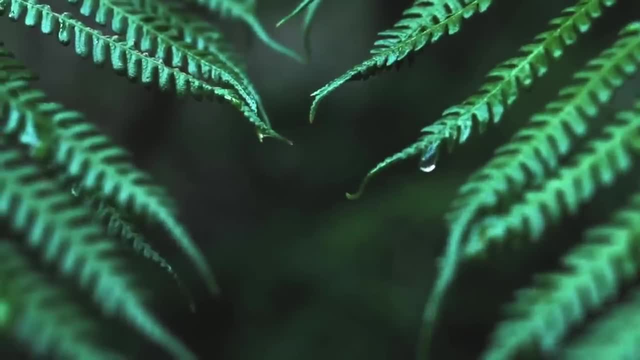 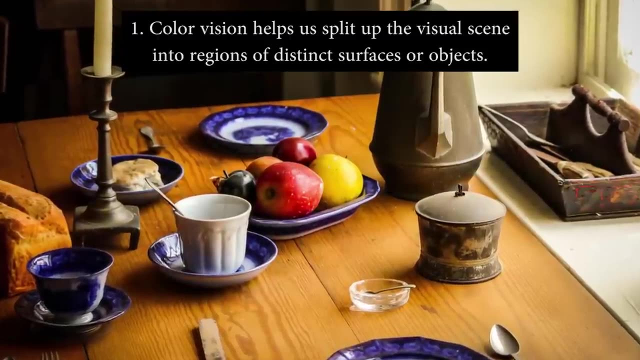 They can show us how ripe a fruit is or how hydrated a plant is. This leads us to Evan Thompson's argument. from perceiver relativity. Color vision helps us split up the visual scene into regions of distinct surfaces or objects. Color vision varies considerably throughout the animal world. 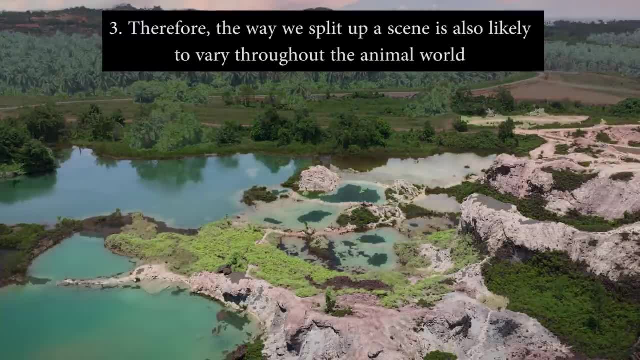 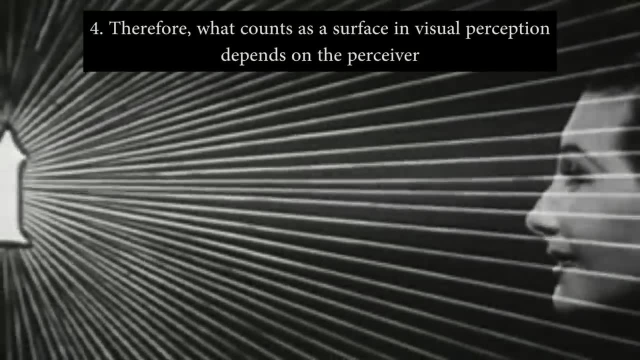 Therefore, the way we split up a scene is also likely to vary throughout the animal world. Therefore, what counts as a surface in visual perception depends on the perception, And that's the perception we've got. All of this makes sense when you consider evolutionary adaptation. 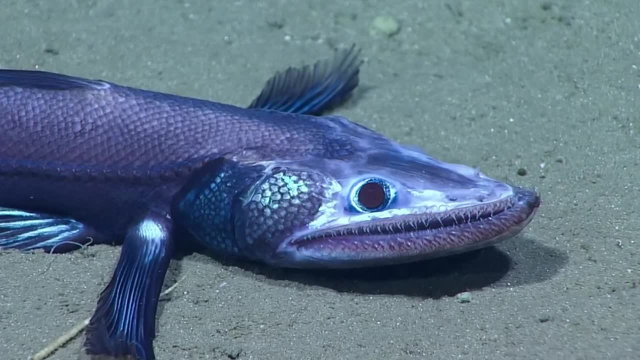 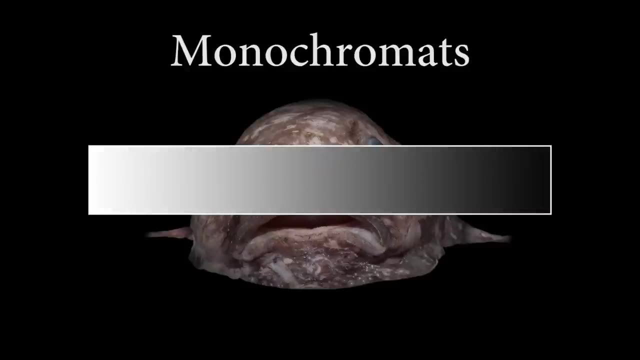 Consider deep-sea fish, for example. When you're that far down in the ocean, things are pretty dark. These creepy little guys are usually monochromats, meaning that they only see the intensity of light, but no color. A lot of them hunt their prey from below. so their light perception is tuned to be sensitive to the maximum contrast to detect movement in their prey. The further up in the ocean you go, where there is much more light around, the fish have much more variety in the colors they're able to perceive. 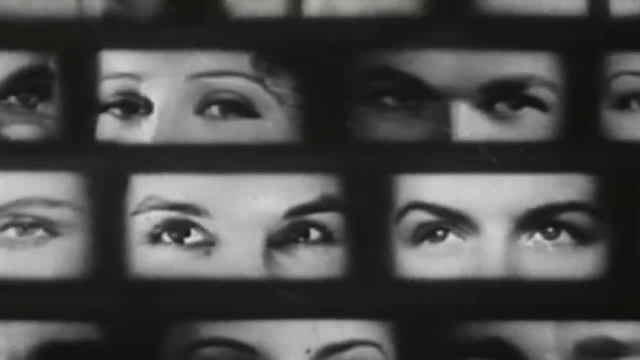 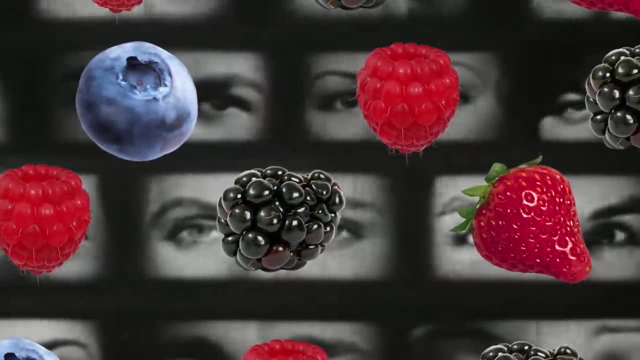 Now what about us humans? Since the 1950s, some people have suggested that the way primate perception is configured actually co-evolved with colored fruits, And recent studies support this view too: Species of monkeys like macaques, patas monkeys and guanons. 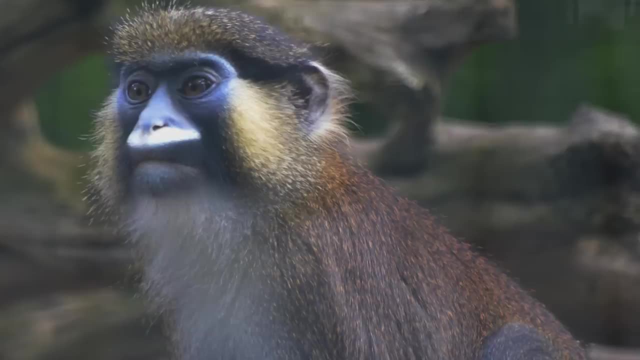 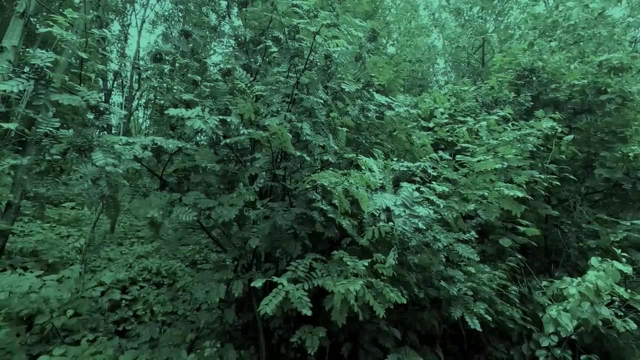 all have similar sensitivities in mid-wave pigment and long-wave pigment. They all look very different and live in very different habitats, but they also all eat a lot of fruit. These fruits conveniently tend to be very brightly colored and stand out in the green foliage.